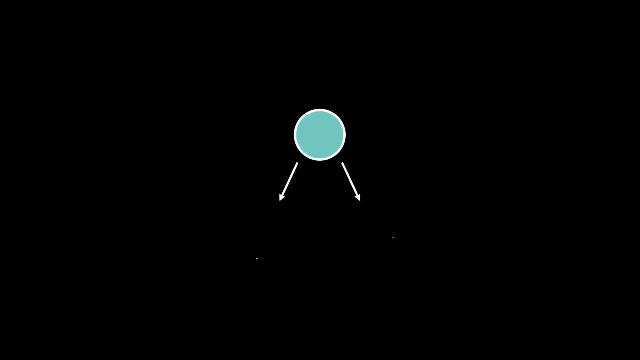 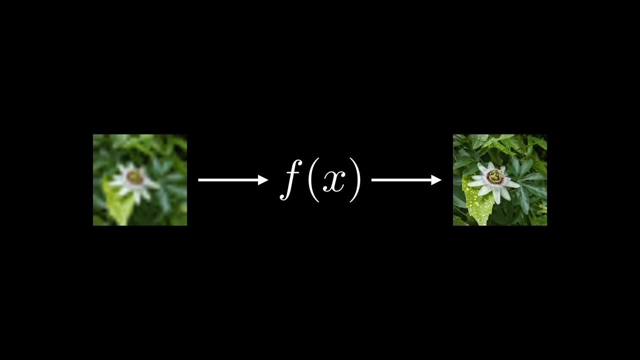 I want you to imagine approximating a function parameterized by a deep neural network. In this example, we're going to pass our network an upsampled, low resolution input image and pass it through each of the network layers. We want the network to output the input image. 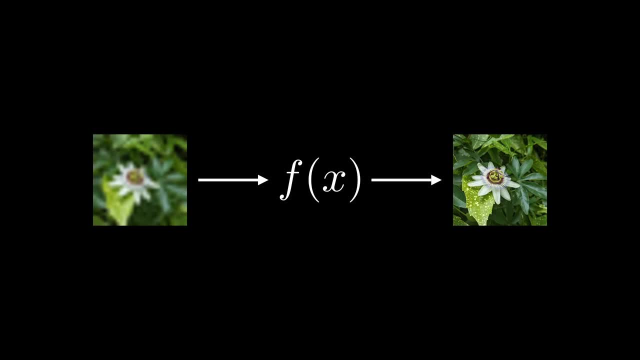 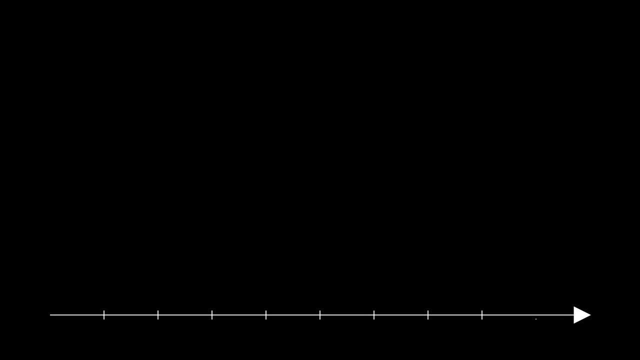 but now in a high resolution, a task commonly known as super resolution. Unfortunately, in practice, after training our network on high and low resolution image pairs, somehow our network is spitting out images that are even worse than our input. After putting all your effort into a beautifully deep architecture, you are horrified to see that. 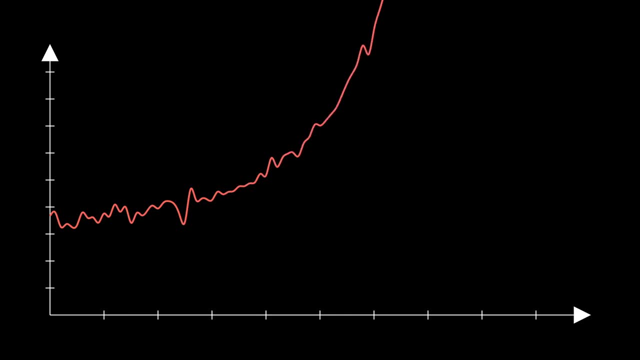 instead of going down, your training loss shoots endlessly upwards. Your classmates and colleagues can't help but laugh. and seemingly counter-intuitive, because now the model has more parameters. Now how can we address this and get your loss going in the right direction? This problem partly comes down to the fact that we have an input signal that is being lost the deeper. 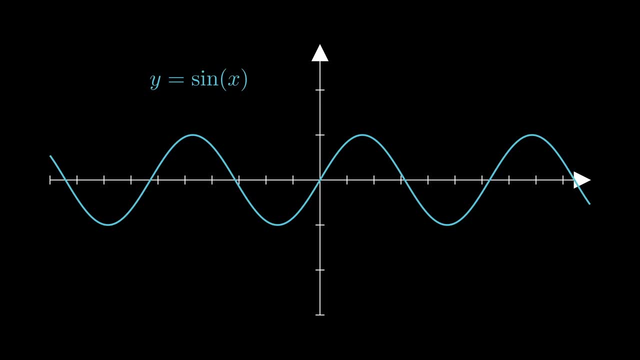 and deeper we go into our network As the signal is passed through each of the non-linear functions at each layer. Look at what can happen to a training signal even after being passed through a single ReLU function, the most popular activation function for neural networks. 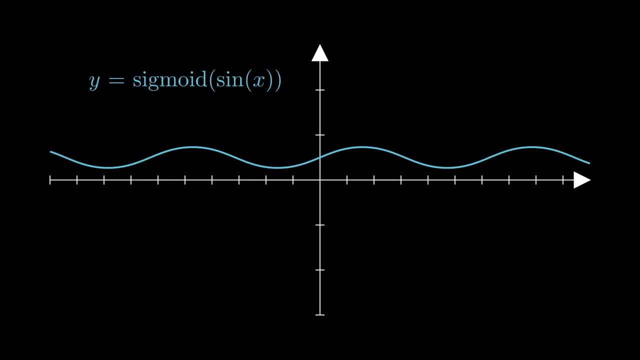 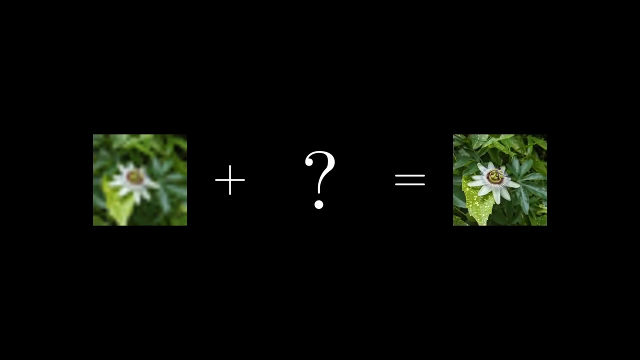 Essentially, you're asking the network to do two things. One is to retain the input signal, and the second is to find out what needs to be added to the input image to transform it from a low to high resolution image. Instead, let's look at the problem from a different angle. Let's first minus the low. 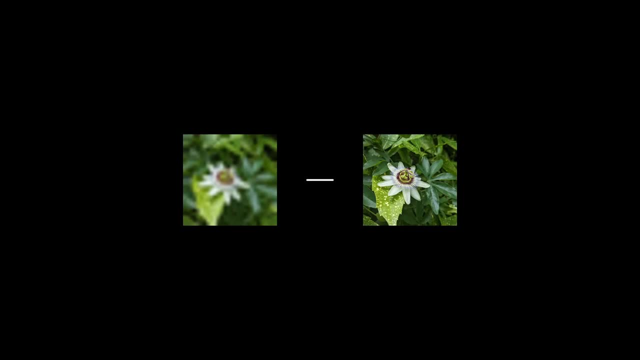 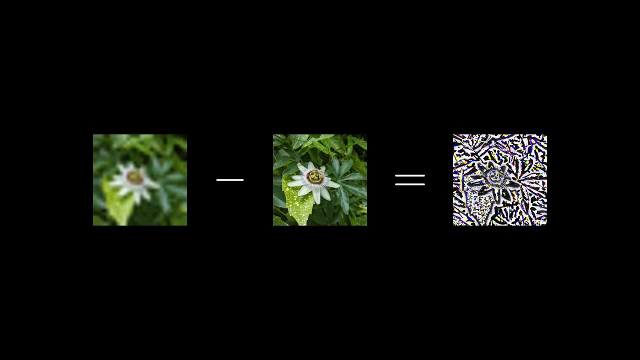 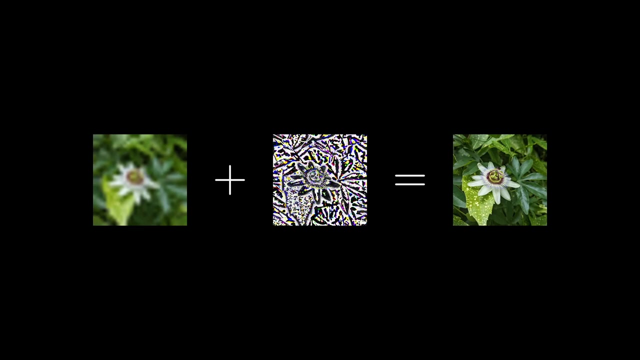 resolution image from one another. This gives us what is known as a residual image, or the difference between the two images. Now let's reshift this equation to get our intended output on the right hand side. Now, given we already have the low resolution image at training time, let's now just 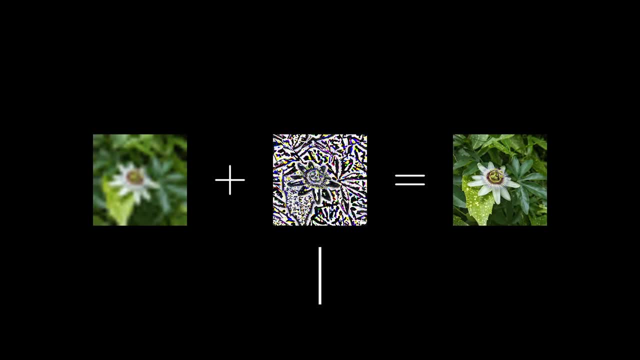 get our network to learn the only bit we actually care about: the residual. Framing the problem in this way makes the network's life easier, as it doesn't need to retain the entire input signal. This was the same intuition that inspired the authors from the 2015 paper. 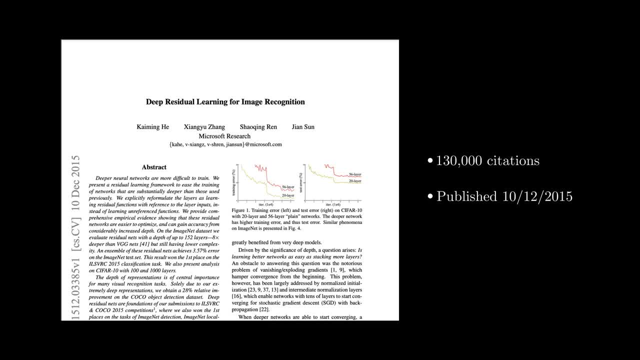 Deep Residual Learning for Image Recognition. This paper is now considered seminal in relation to deep learning, with over 130 000 citations. It is rare to run into a model architecture in deep learning today that doesn't utilize the contributions from this paper in some fashion. 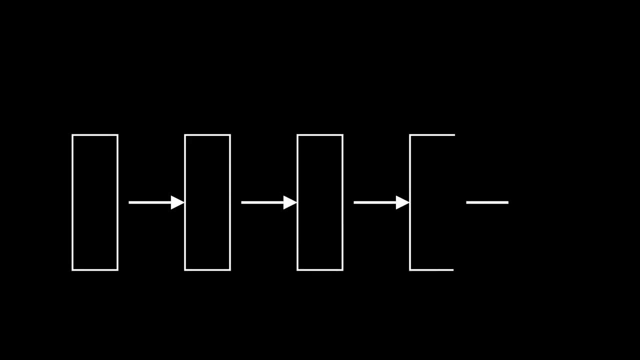 In the previous example, I gave you an easy and intuitive introduction to residuals. Let's have another look at the layer of a neural network. I chose to present residual connections to you using the example of super resolution, as it can be visualized very easily By simply adding. 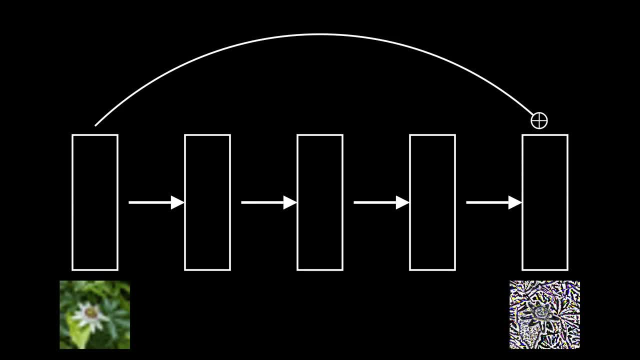 the input onto the output. we can instead learn the mapping to the residual image, as you can see here. However, this approach I've shown you so far has two major problems when generalizing to other tasks. The first problem is where we have a task where the input and outputs don't share. 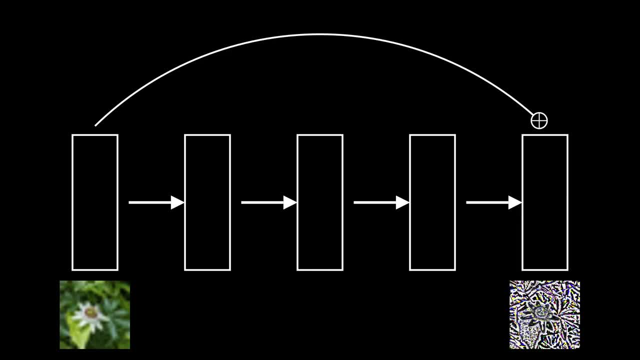 the same dimensionality, For example in image classification, where you take an image input and map it to a single class label. How would you meaningfully add the inputs and outputs in this scenario? The second problem is how the input signal is propagated throughout the network. 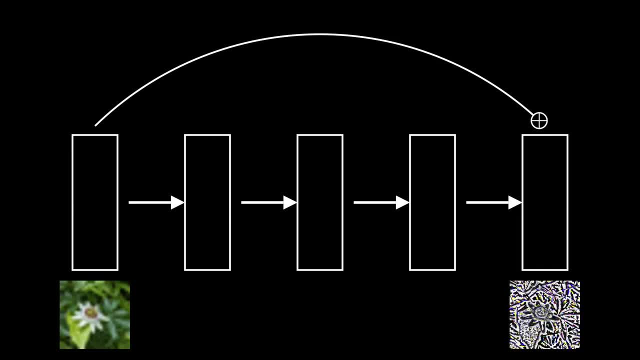 Let's consider the midpoint of our super resolution network. At this point, no matter what our input or output is, it is still easy for the network to lose the training signal. This signal is an important piece of information that would be useful for the network to have access to. 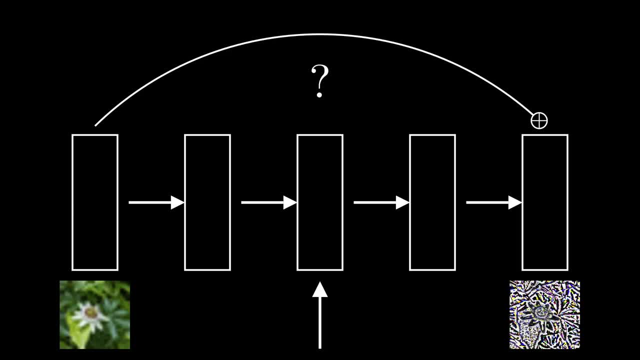 In order to remedy both these problems, we can add what are known as residual connections all the way on our network. This not only boosts input signals all the way along the network, but also makes it easier to submit inputs and outputs. as feature, dimensionality is adjusted. 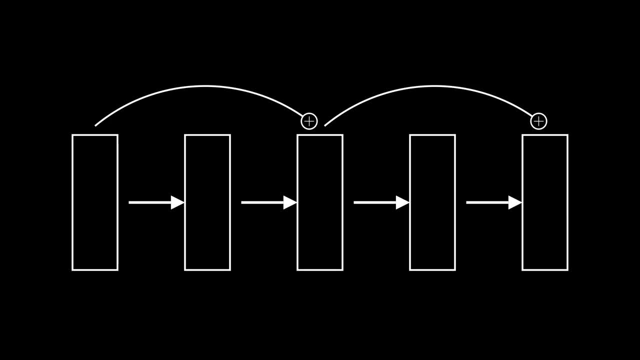 on the go. We can now also view the network as a series of residual blocks instead of a series of independent layers. Most importantly, now the network has the option to not fully use all the blocks, as it is easy stop using the box as the result of almost nothing factoring them Since it. 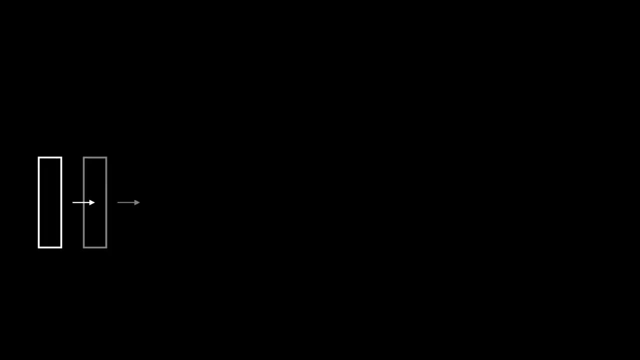 is really fácil de adaptar todas las llamas desde el intento de eliminar enough de diferentes, since it is easy for each block to output the identity function and take no penalty in relation to the loss function. This opens the doors to training extremely deep networks. 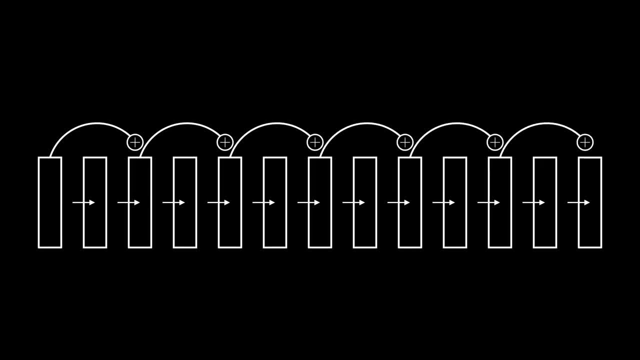 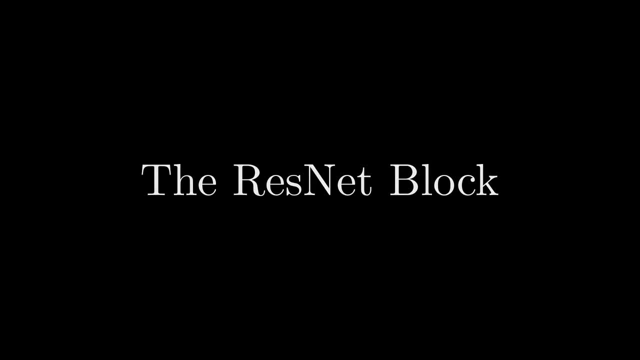 Now let's have a deeper look at the main idea I introduced here: the residual block. So what exactly was the ResNet block they proposed in the original paper? Let's go through it step-by-step. Firstly, we pass our inputs through a 3x3. 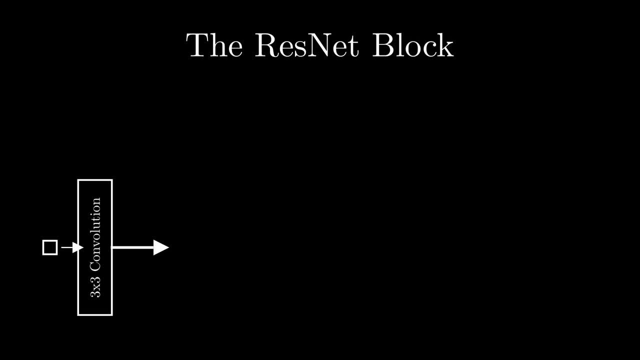 convolutional layer with a stride of 1 and padding 1.. These parameters mean that our output features will have the same dimensionality as our input. We then apply batch norm to renormalise these features and pass them through an activation function such as ReLU. 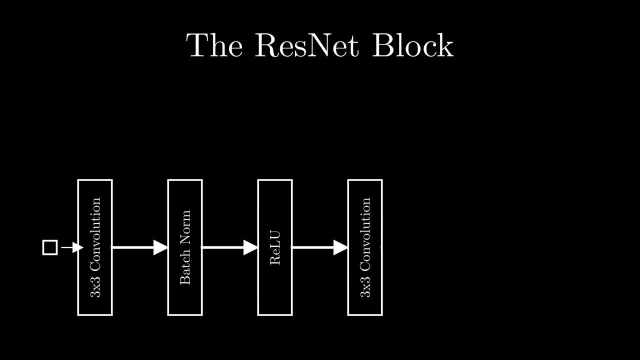 We then pass the features through a second convolutional layer, the same as the first, and again followed by a batch norm. At this stage we just have a normal vanilla neural grey frame based on the срав nochl and reneg behave by spiritual analysis. 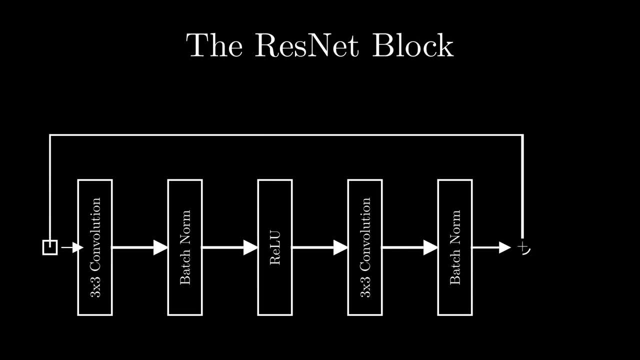 network. so let's now add a residual connection. we can do this by simply adding the blocks inputs onto the current set of features. we do this element wise, as our inputs and features share the same dimensionality. remember this is only because we have carefully chosen our convolutional parameters. 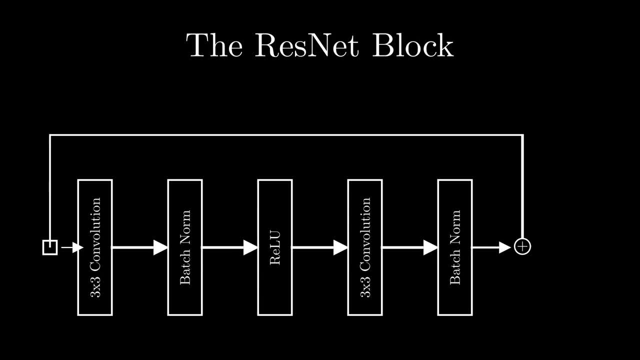 however, for tasks such as image classification, we do actually want to reduce our dimensionality throughout the network. more on that in a moment. finally, we pass our features through a final activation function. now, that is essentially it. it really is quite a simple idea. now let's have a quick look. 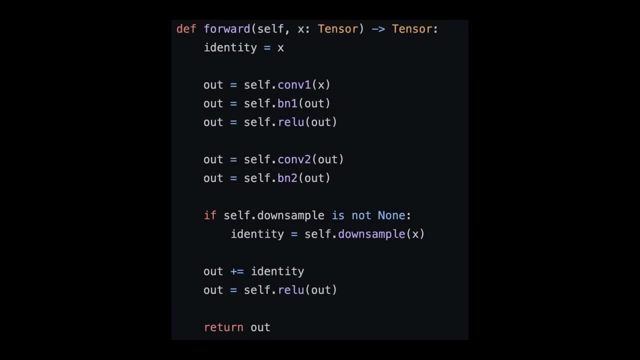 at the official pytorch code implementation for a ResNet blocks forward, pass and consolidate what we've just learned. we start with an input, tensor X, and save a copy of this as our identity function we can use later. we then pass our input through a set of convolutional batch norm and activation. 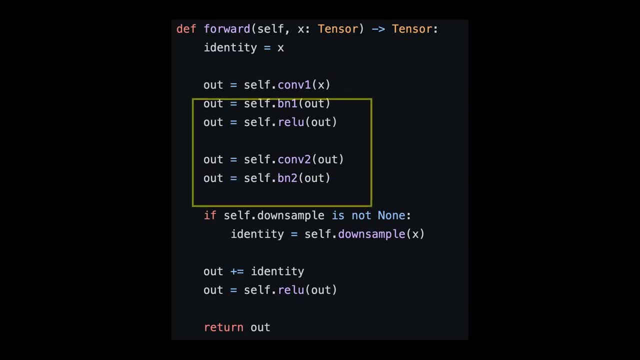 layers down, sampling the features if required. more on that a moment when we discuss dimension matching. we can then simply add our saved identity features to our current set of features in the network. you can then simply add our saved identity features to our current set of features in the network. 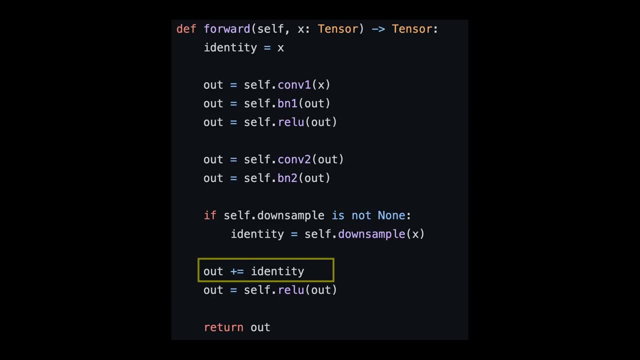 this is done element wise. finally, we pass this through a final activation function and return this as the output of our residual block. note that some of these choices are arbitrary, such as applying the activation function after adding the identity function. this is simply done because this is what the 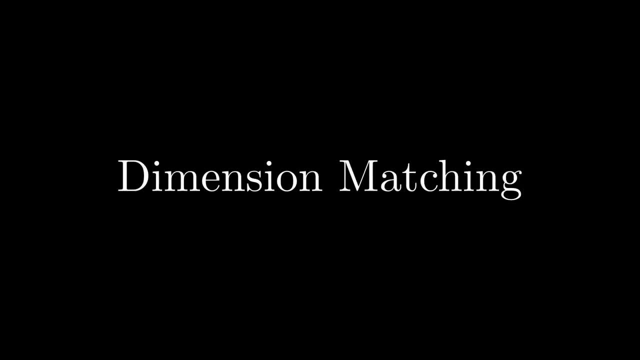 author has found to give the best results when performing a residual connection, we must ensure that the dimensions match such that we can do element wise addition. in the original paper they choose to reduce dimensionality every few residual blocks and then we can add our set of features. 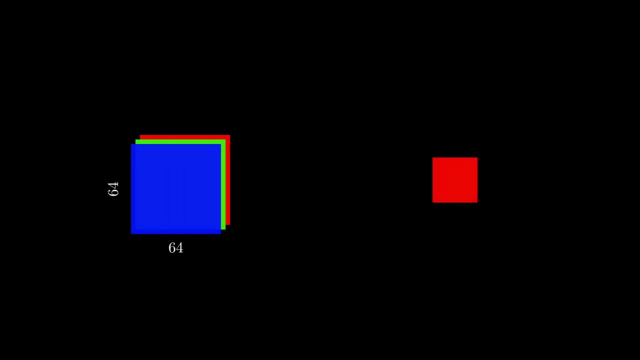 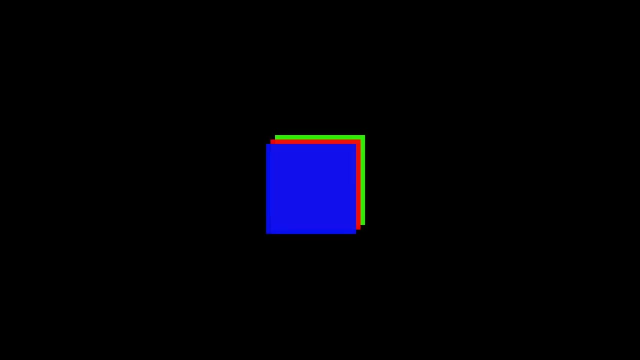 as their end goal is image classification, where you go from a high dimensional input to a low dimensional output, the authors decided to reduce dimensions by halving the height and the width of their current set of features to keep the computational requirements of each part of the network. 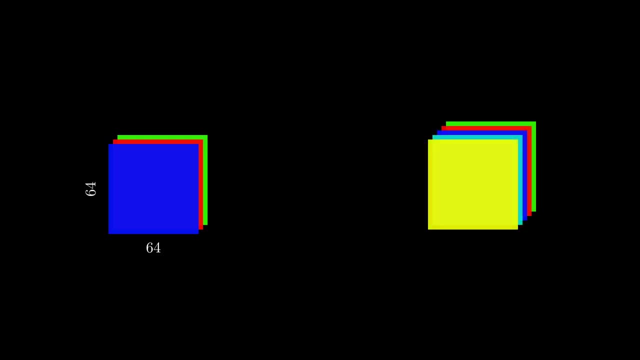 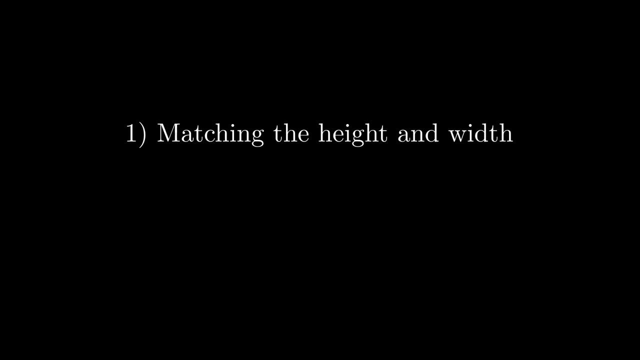 consistent. they also increase the number of channels every time they half the height and the width. this leaves us with potentially two scenarios of mismatched dimensions: firstly, where the height and the width don't match, and secondly, where the channels don't match. it could be either. 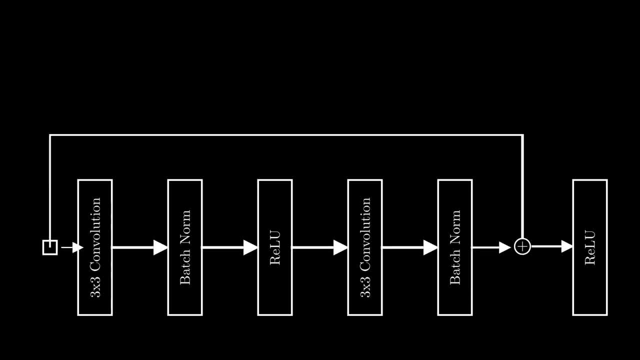 one of these or a combination of the two. Let's have another look at the ResNet block and understand how the network can downsample features. Let's have a look at the first convolution which I told you earlier had a stride of one and padding of one to keep input feature dimensionality the same as 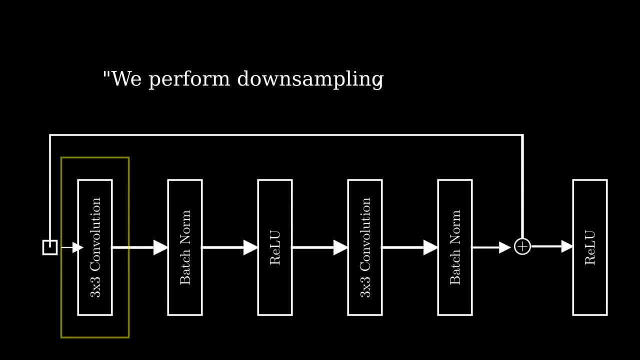 the output. The authors proposed to downsample features directly by occasionally altering this convolutional layer to have a stride of two. This produces features with half the height and half the width. When the authors downsample in this fashion, they also double the number of convolutional 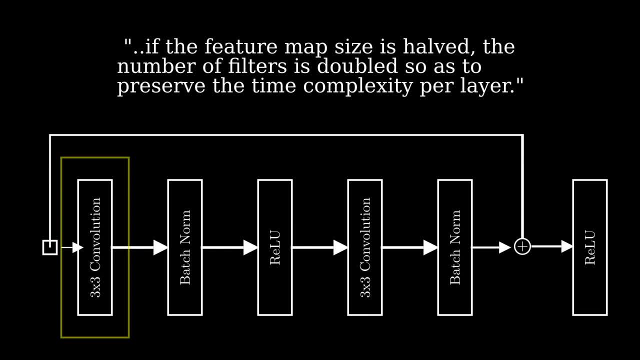 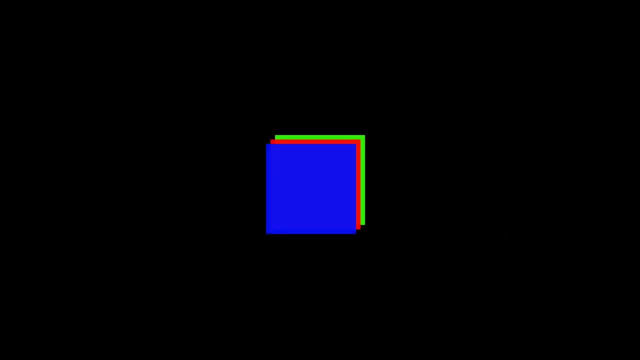 filters, which in turn doubles the number of channels in the output features. This is where we have a problem with dimension matching, as our input that is sent through our residual connection does not have the same dimensions as the features coming through our network. Let's now have a look at our input features coming through our residual connection. 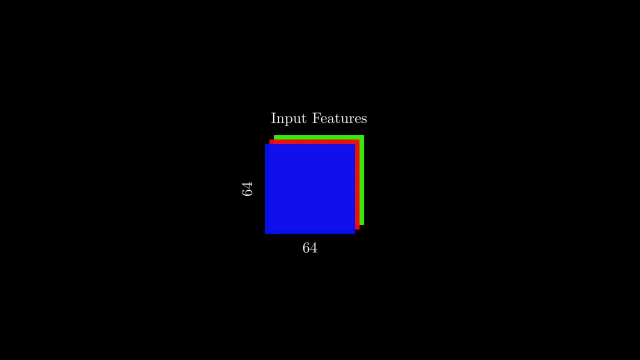 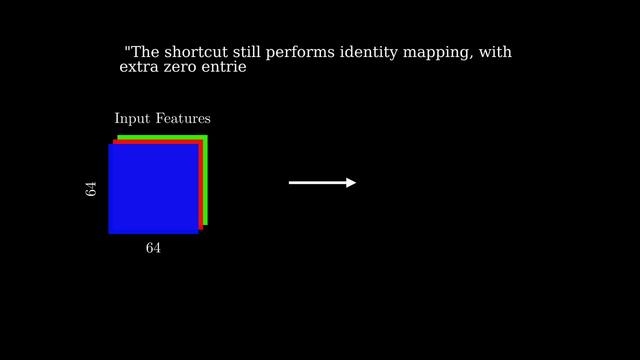 and see what options are available to us when addressing this dimension mismatch. The authors proposed two solutions. Firstly, they propose to match the number of feature channels by zero padding. This option has the benefit of introducing no new parameters into the model. This is simply done by filling up half the features with zeros, Although no parameters. 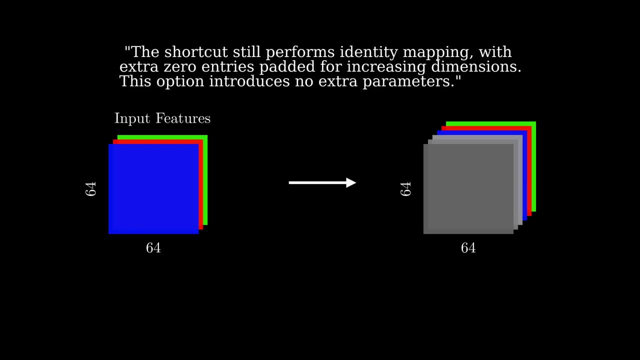 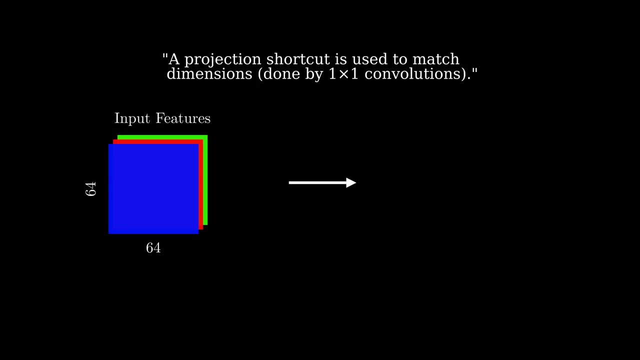 are added. we are now wasting computation on meaningless features full of zeros. The second solution is to match the number of channels by passing over our input features with a one by one convolution. This of course, adds extra parameters. that means there are only three channels in our output features. So, for example, if our input features had three channels?